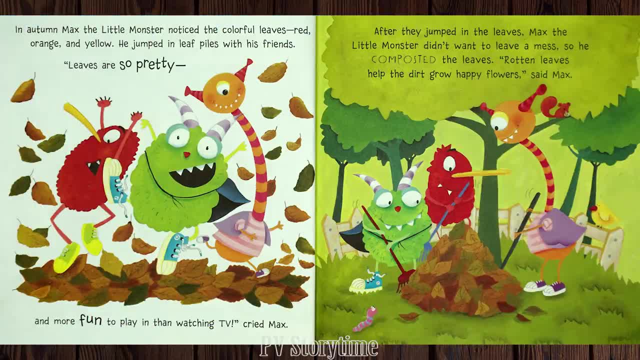 In autumn, Max, the Little Monster, noticed the colorful leaves- Red orange and yellow, Red orange and yellow, yellow. He jumped in leaf piles with his friends. Leaves are so pretty and more fun to play in than watching TV, cried Max. 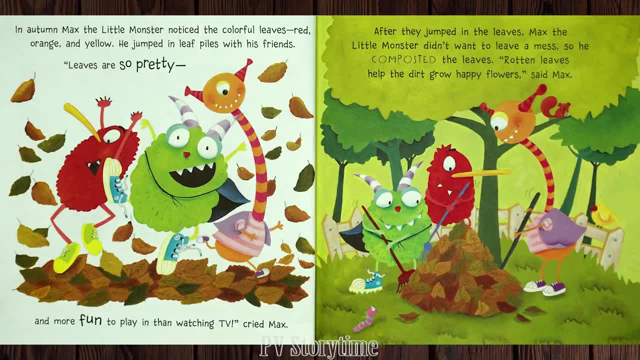 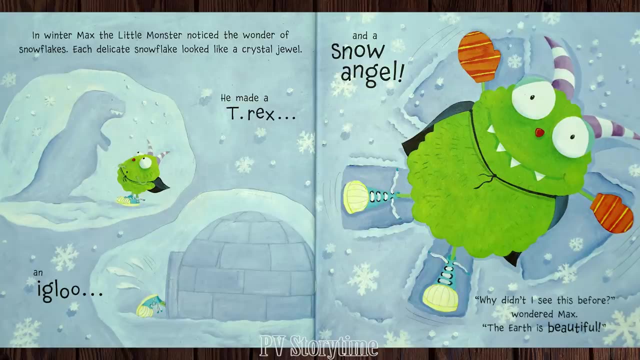 After they jumped in the leaves, Max the little monster didn't want to leave a mess, so he composted the leaves. Rotten leaves help the dirt grow, happy flowers, said Max. In winter, Max the little monster noticed the wonder of snowflakes. 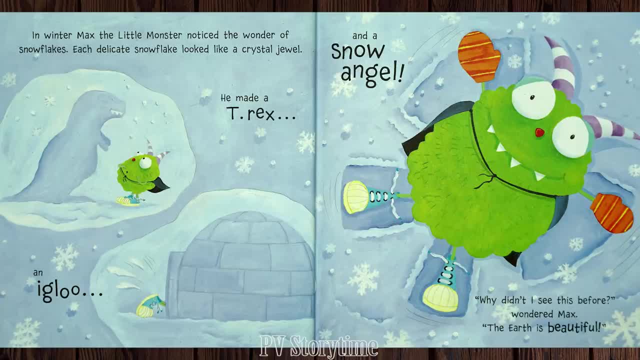 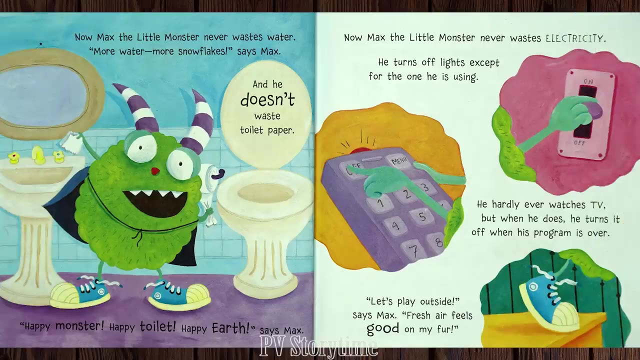 Each delicate snowflake looked like a crystal jewel. He made a T-rex, an igloo and a snow angel. Why didn't I see this before, wondered Max. The earth is beautiful Now. Max, the little monster, never wastes water. 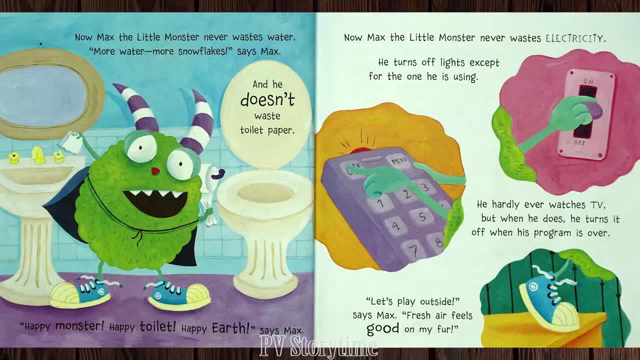 More water, more snowflakes, says Max, And he doesn't waste water, He doesn't waste toilet paper. Happy monster, happy toilet, happy earth, says Max. Now, Max, the little monster, never wastes electricity. He turns off lights, except for the one he is using. 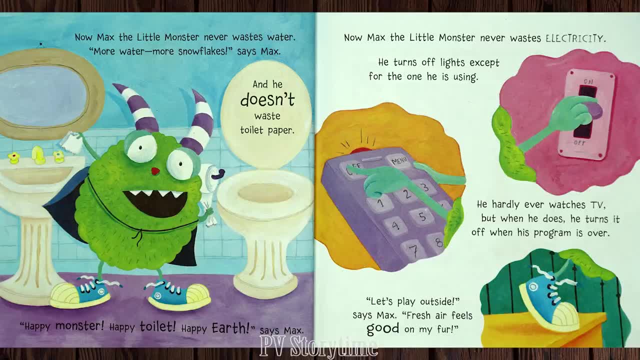 He hardly ever watches TV, but when he does, he turns it off. when his program is over, Let's play outside, says Max. Fresh air feels good on my fur Now. Max, the little monster, never litters. He doesn't waste water. 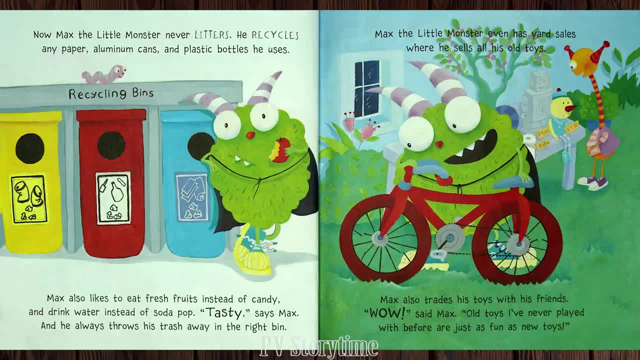 He recycles any paper, aluminum cans and plastic bottles he uses. Max also likes to eat fresh fruits instead of candy and drink water instead of soda pop. Tasty, says Max, and he always throws his trash away in the right bin. 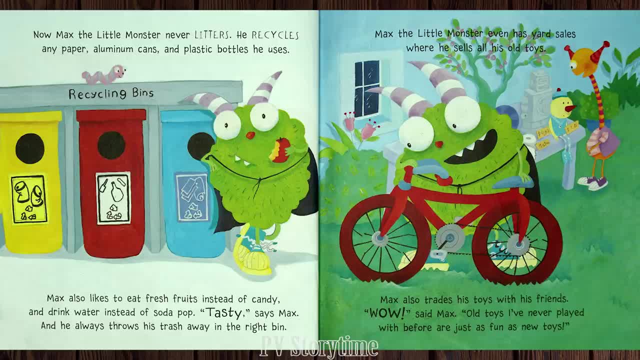 Max the little monster even has yard sales where he sells all his old toys. Max also trades his toys with his friends. Wow, said Max, Old toys I've never played with before are just as fun as new toys. Now, Max the little monster loves the earth. 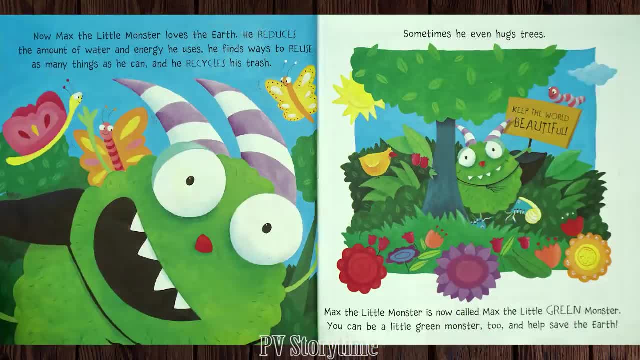 He reduces the amount of water and energy he uses. He finds ways to re-use as many things as he can and he recycles his trash. Sometimes he even hugs trees. Max the little monster is now called Max the little green monster. He is a bit more of a child than his old friends, but he is a little naughty.